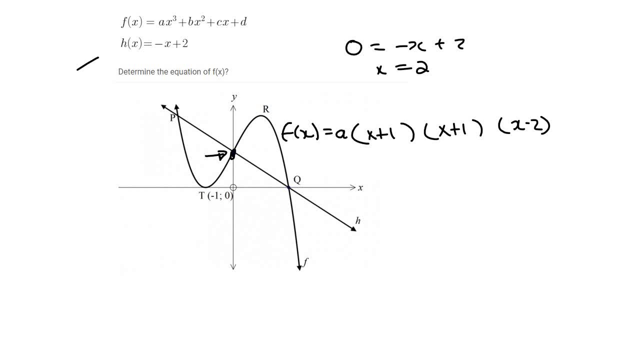 So we could find this point over here, Because it's the interception of the straight line with the y-axis and we have the straight line's equation. So we can make x 0 like that and that's going to give us 2.. 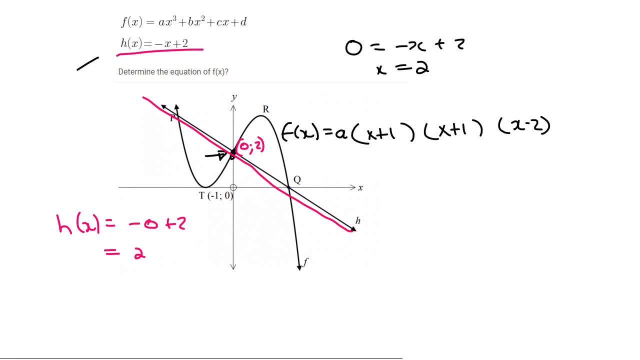 So the coordinates here would be 0 and 2.. But luckily that point is also on the cubic graph and so we can use it to find a. So we can say: 2 equals to a 0 plus 1, 0 plus 1, 0 minus 2.. 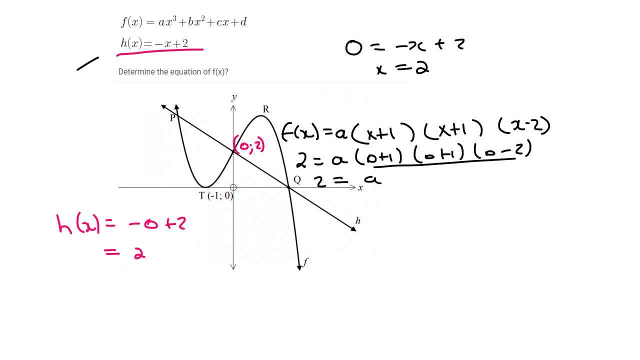 And so that's going to be: 2 equals to a. All of these numbers multiplied together is just going to be minus 2, and so a would equal minus 1.. And so now I can say f of x equals to minus 1, then I can put the brackets x plus 1, x plus 1,, x minus 2.. 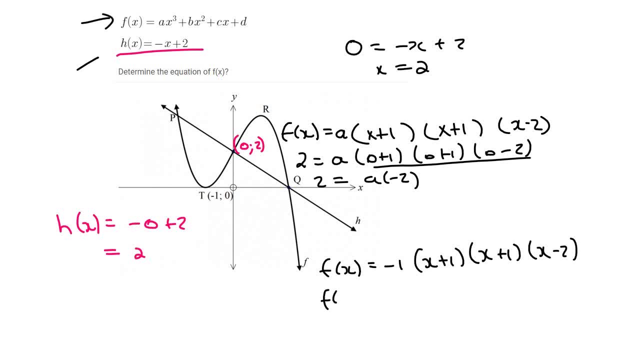 To make it look like f of x, I would have to multiply everything out. So I'm going to leave the minus 1 in the front and I'm going to multiply these two together. That would give me x squared plus 2x plus 1.. 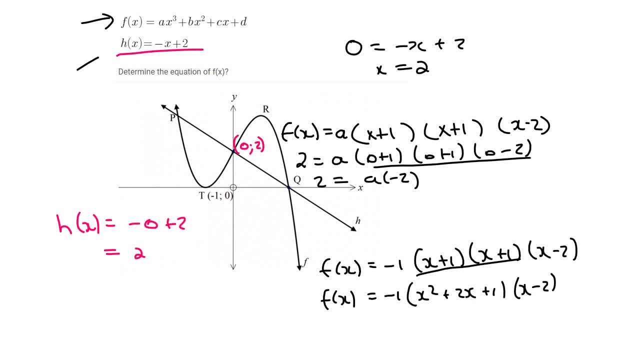 And then I've still got an x Minus 2.. Next I'm going to- So I'm just multiplying everything out- You guys know how to do this- And then I'm going to put the minus 1 into that. 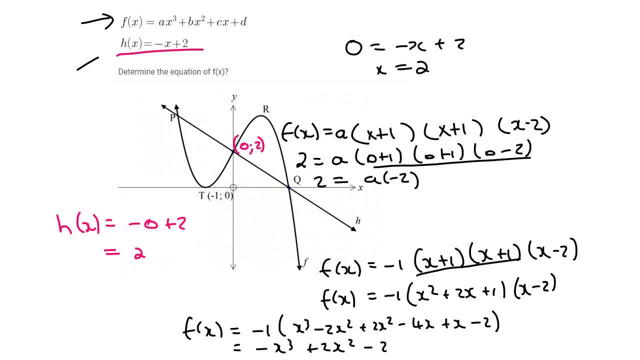 So that'll be minus x cubed plus 2x squared, minus 2x squared plus 4x, minus x plus 2. Then you can just simplify all the like terms And that's going to be minus x cubed. Those cancel out. It's going to be plus 3x plus 2.. 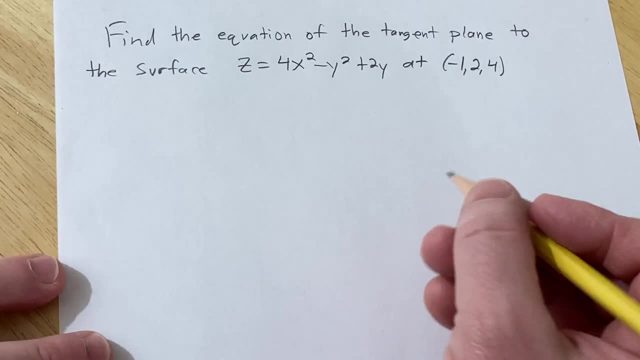 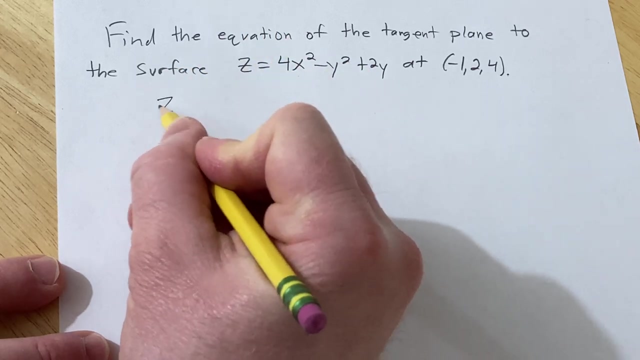 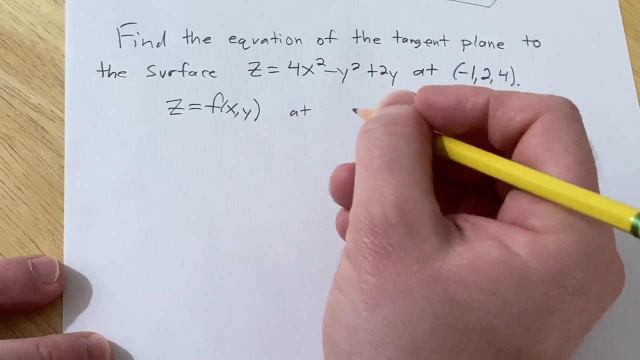 Find the equation of the tangent plane to the surface z equals 4x squared minus y, squared plus 2y at negative 1 to 4.. So to do this we are basically going to use a formula. The formula says: if you have a surface z equals f of x, y and you want the tangent plane at, say, p, x, naught y.